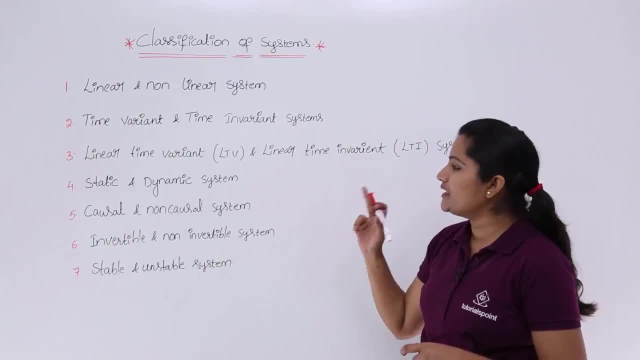 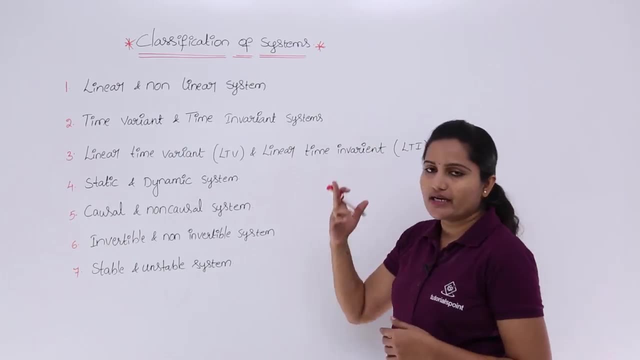 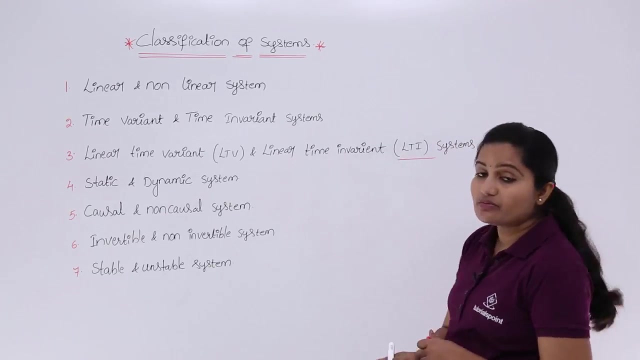 to be linear time variant system. and here coming to linear time invariant system, if a system satisfies the condition of linearity and time invariance, then that particular system is said to be linear time invariant system. Particularly this LTI ATI systems are very, very important for our signals and systems point of view. 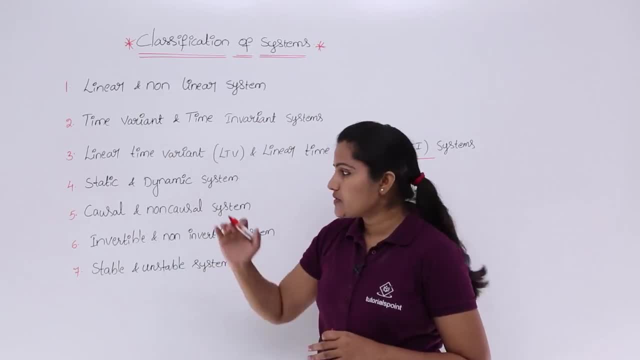 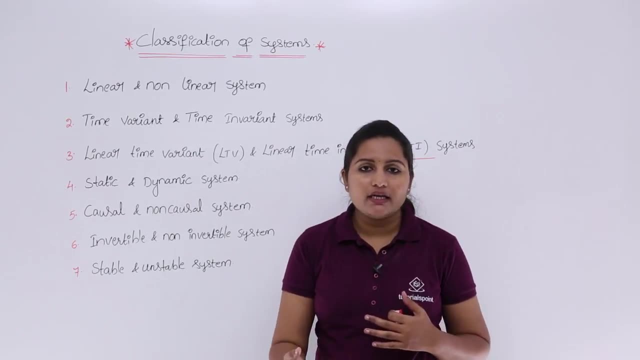 So now coming to static and dynamic system. So static system is a memory less system which stores whatever we are giving now. So dynamic system is having memory and it is having some knowledge on previous inputs and outputs also. So simply we can say static system is a memory less system and dynamic system is a memory system. 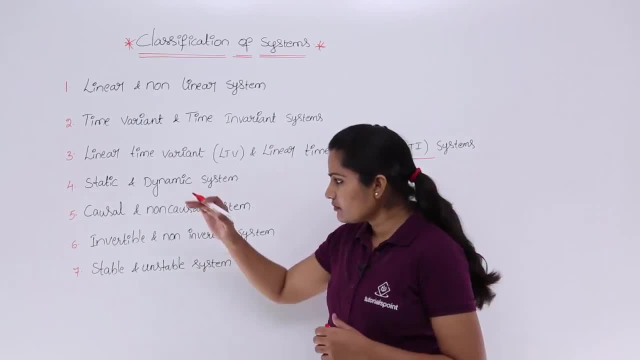 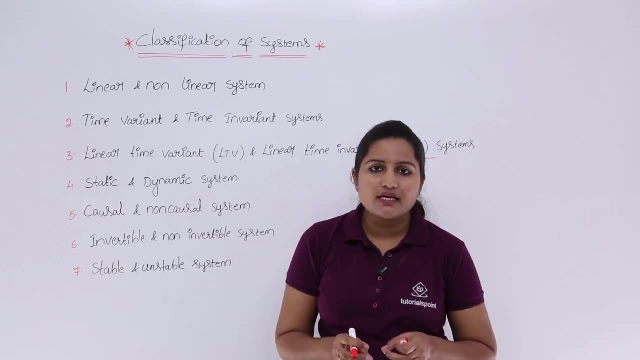 So, coming to causal and non-causal system. causal system, the characteristics of the system, the system response will depends upon the present and past inputs. So here, non-causal system, so which is not obeying that causal system feature, that is called as non-causal. 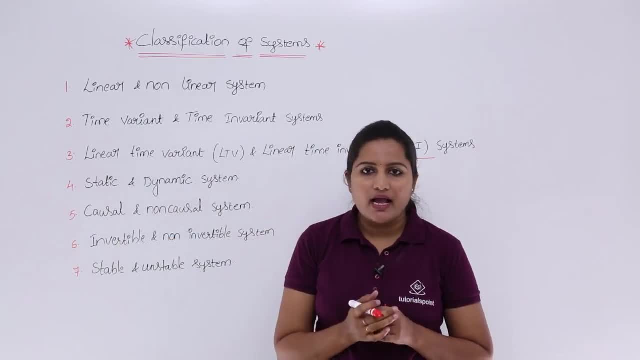 So here, whatever inputs we are having, that means if a system response Response is depend upon only present and past, that is said to be causal, otherwise non-causal. So now coming to invertible and non-invertible system, If a system response is invertible, that means if you are having a system internal to any system that is, that can invert the response to its actual, then that is called as invertible system. 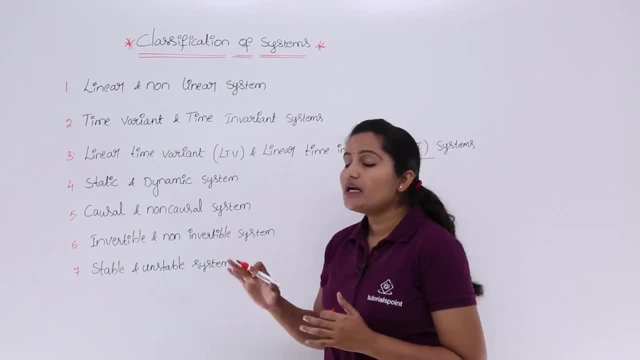 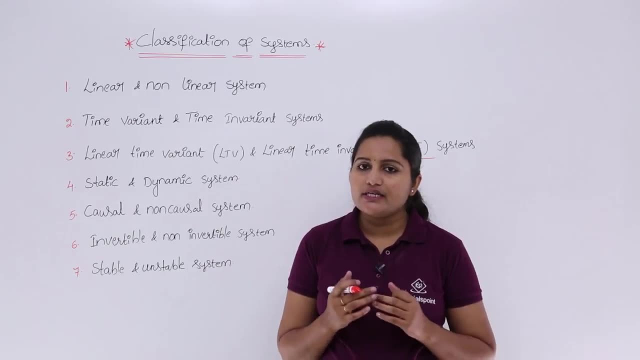 Otherwise that is called as non-invertible system. So here, finally, we are having stable system and unstable system. So for A system is said to be a stable system when for a bounded input, if that is producing bounded output, then that is said to be a stable system. 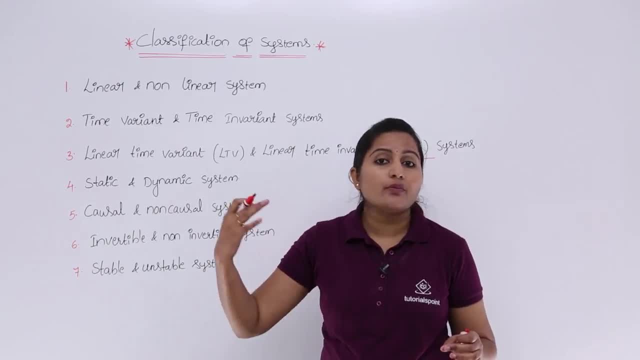 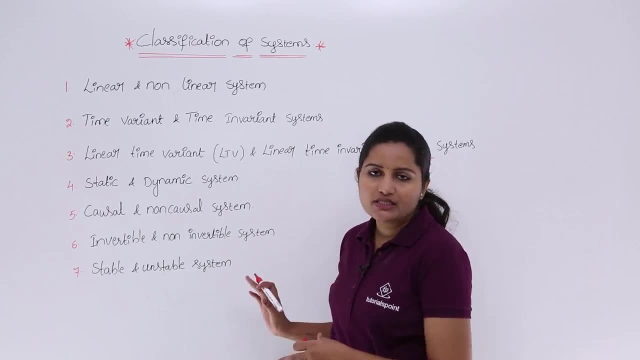 For a bounded input. if it is producing unbounded output, then that is called as unstable system. Each and every classification of these systems we will discuss one by one, from next class onwards. that means linear and non-linear time, variant, invariant, LTI and LTV. 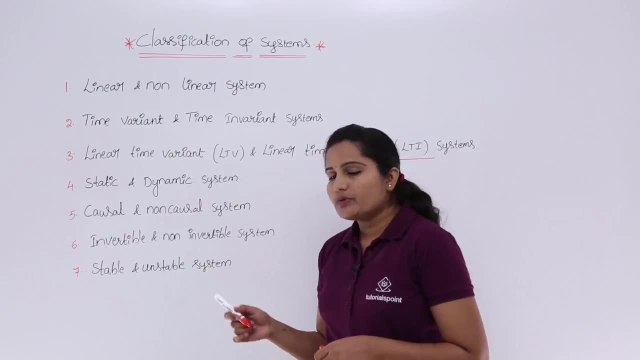 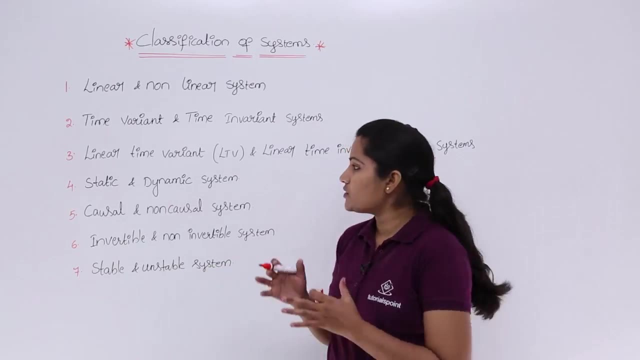 And static and dynamic, causal and non-causal, invertible and non-invertible, static and unstable, stable and unstable system. So we will discuss one by one, from next class onwards, with some examples.